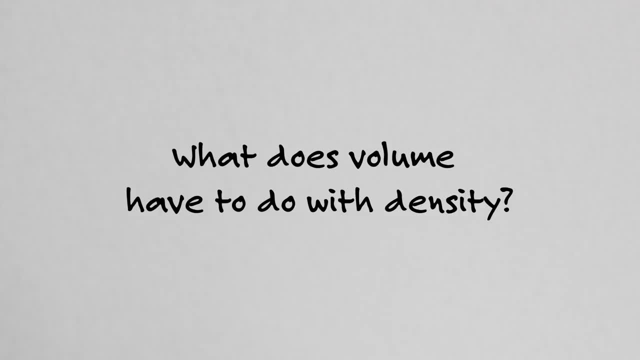 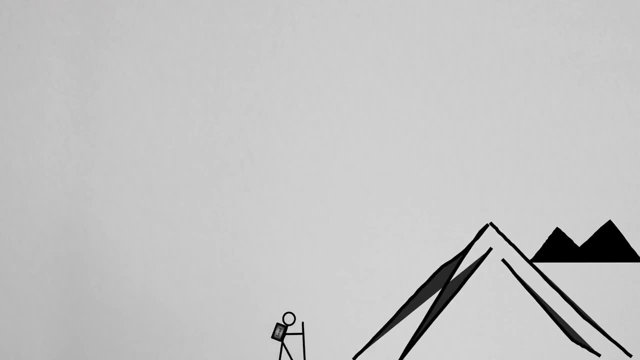 What does volume have to do with density? Quite a bit, actually. Density is how much mass of a substance you can have in a volume. We notice different densities almost every day. I suspect you would be more willing to carry a block of Styrofoam up a mountain than an equal volume of 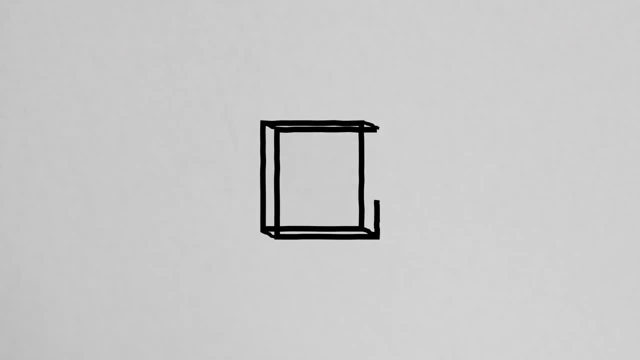 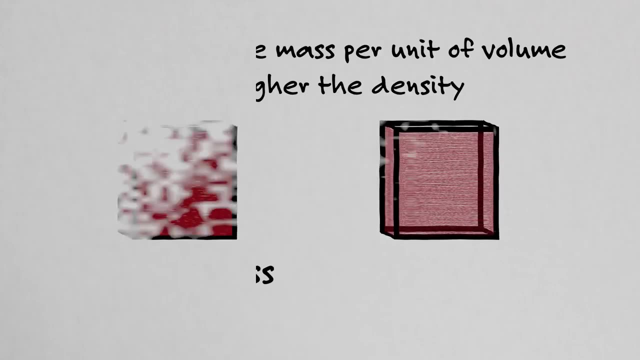 lead. You can have a large object with very little mass or the same size object with a large mass. The higher the mass per unit of volume, the higher the density. So if density is the amount of mass in a volume, then dividing the mass of a substance by its 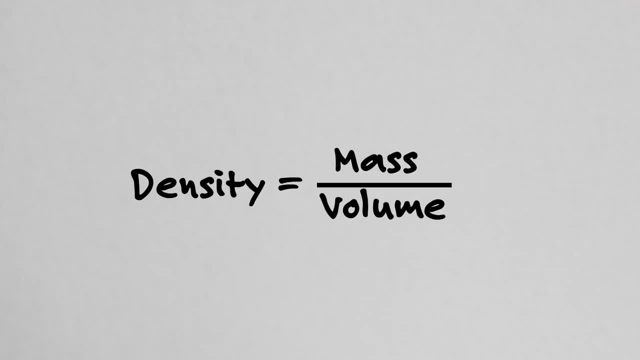 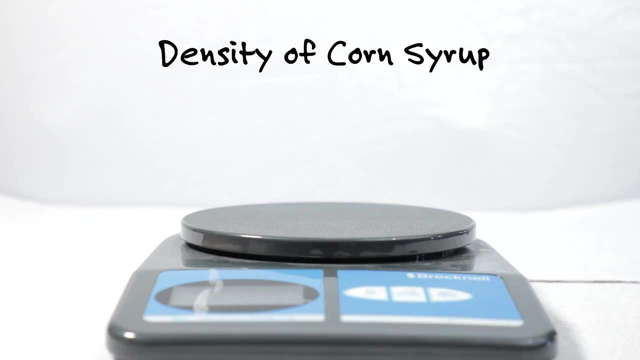 volume tells us how much mass is contained in one unit of volume. The official equation is: density equals mass divided by volume. Let's see how this works with an experiment. To calculate the density, we need to know the mass and volume of our corn syrup. 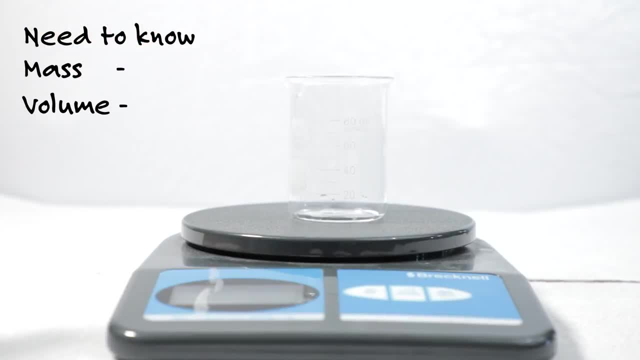 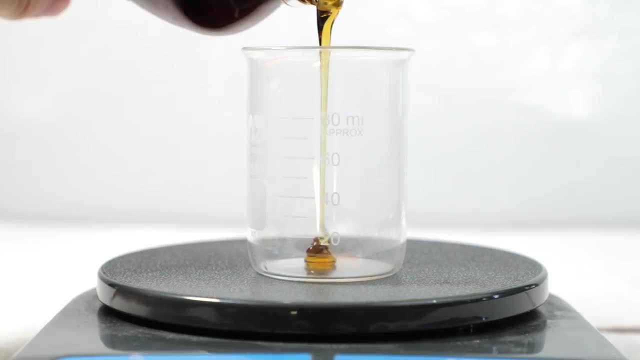 So let's first measure out the mass of our container, since we are only interested in the mass of the syrup. My beaker weighs 48 grams. Now I will measure out 20 milliliters of corn syrup. The scale gives us the total mass of corn syrup. 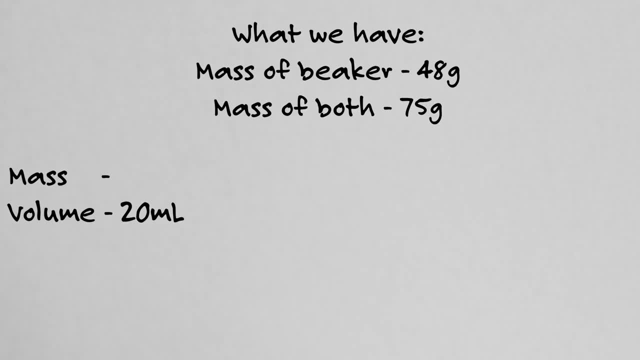 Time for some math. We subtract the mass of the beaker from the mass of the beaker containing corn syrup. We do not want the mass of the container in the calculation, So we subtract and that gives us a difference of 27 grams. To calculate density we take some of the mass of the syrup, which is 27. 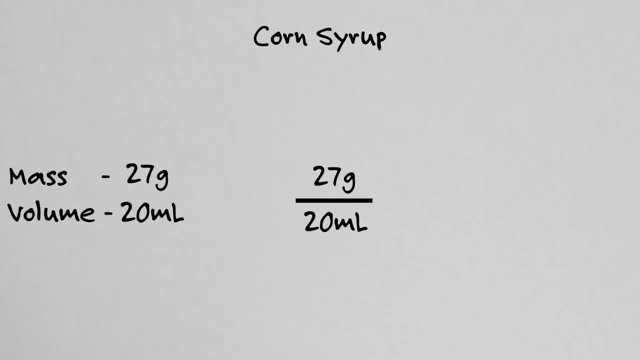 grams and divide that by the volume of 20 milliliters, We do the math and we get a resulting density of 1.4 grams per milliliter, rounded to two significant figures. What that means: for every milliliter of volume I have 1.4 grams of corn syrup. 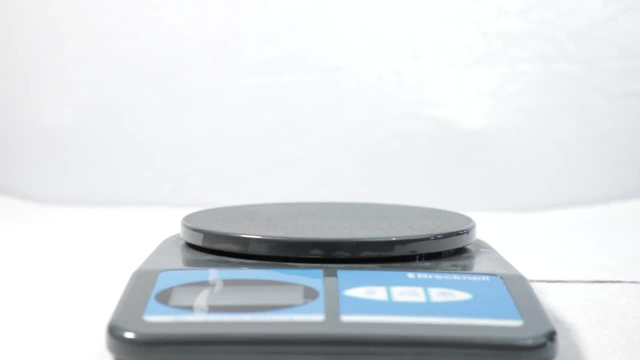 Let's do another calculation, this time using water. If you have a digital scale, the easy way to get the mass of an object minus the container is to use the tare function. Place the container on the scale and then press tare. Now add 20 milliliters of water to the measuring cup. 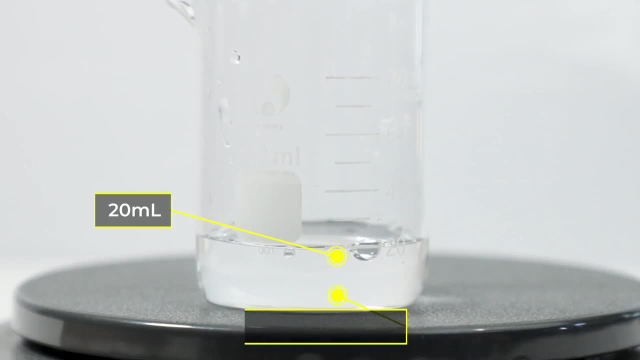 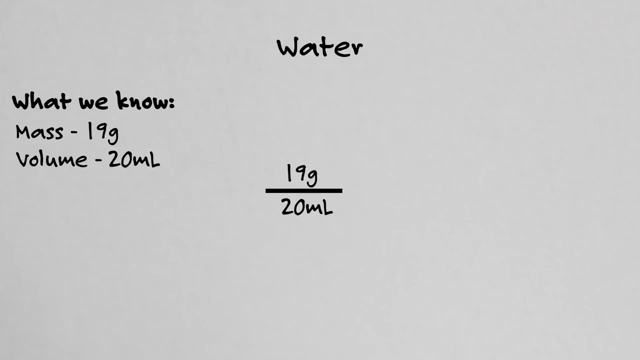 This is our volume. The scale does the work and gives us the mass of water, and I have 19 grams To calculate the density of this soil. we divide 19 grams by 20 milliliters and that gives me a density of 0.95 grams per milliliter. That rounds to 1.0 grams per milliliter As a side note.